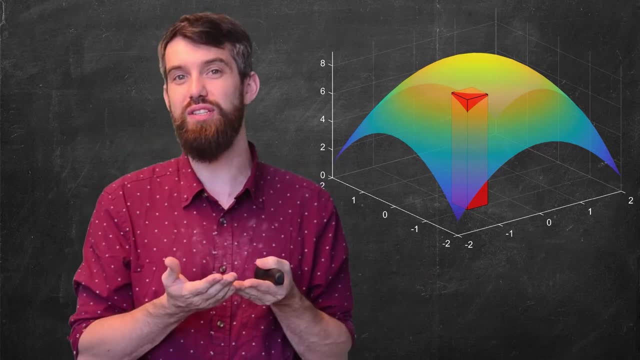 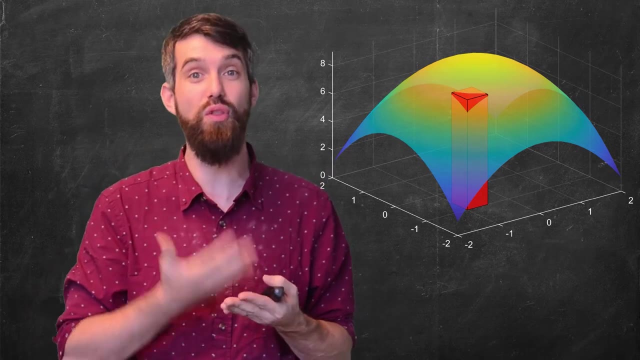 you're adding up too much, and when it's beneath the surface, you're adding up a little bit too little. But as you increase the number of them, as the size of these get smaller. the argument is that these errors, by approximating in this way, 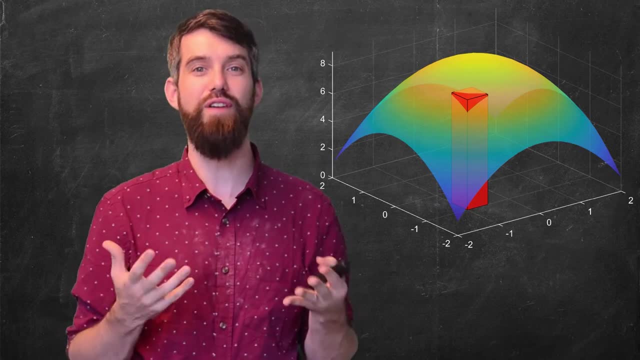 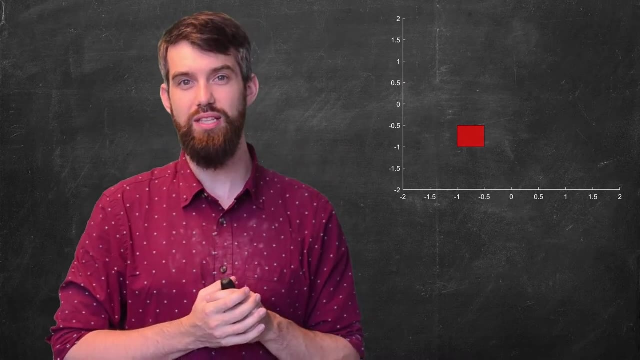 are going to get smaller and smaller and smaller. Let's see how we can define this a bit more formally. I'm going to focus in just on the domain and I've specified some rectangle in the domain. This rectangle has a width that I will define to be delta x. 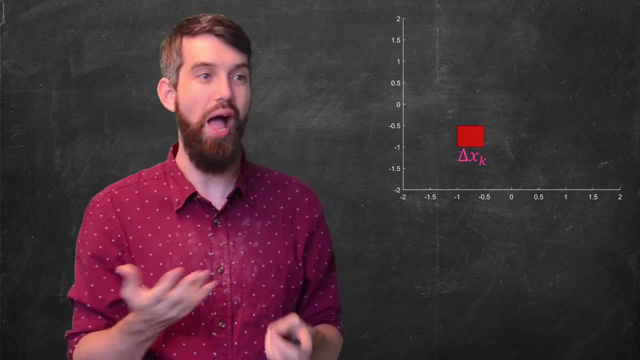 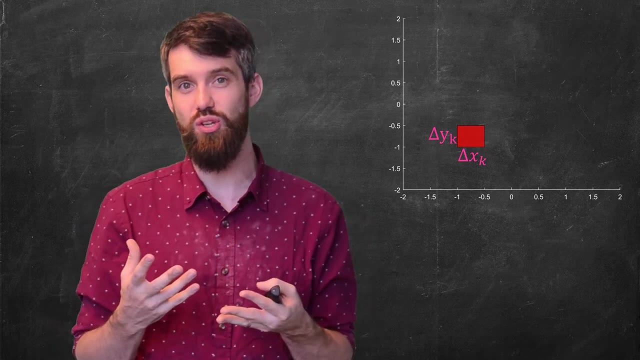 and it has a height change, a delta y, and I'll define that to be the delta y. I'm imagining that there's going to be a large number of these little rectangles subdividing up the domain, and so I actually call it delta x k and delta y k didn't open. 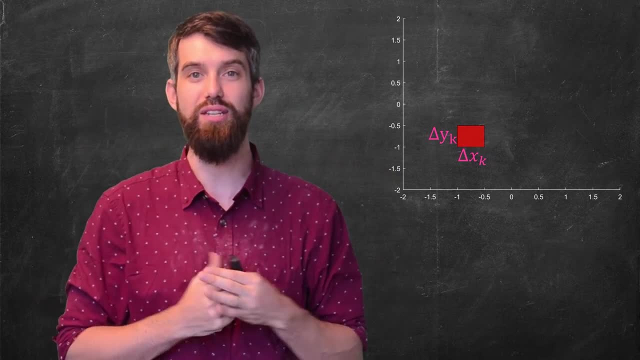 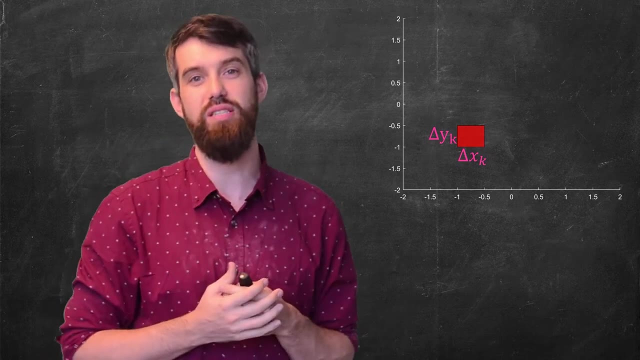 I'm talking about the kth, such little rectangle in the division of my domain. And then the next thing I want to do is I need to figure out what the height of the box is above this little rectangle, and to do that I'm going to plug it into my function. 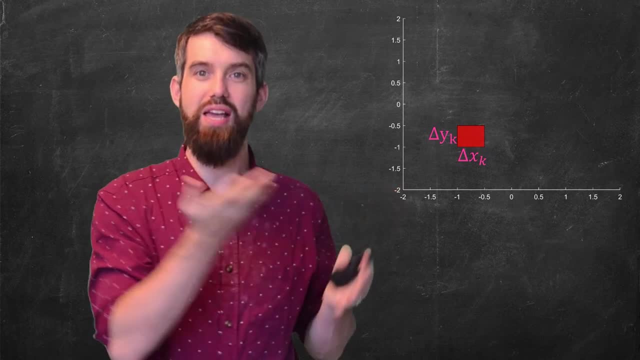 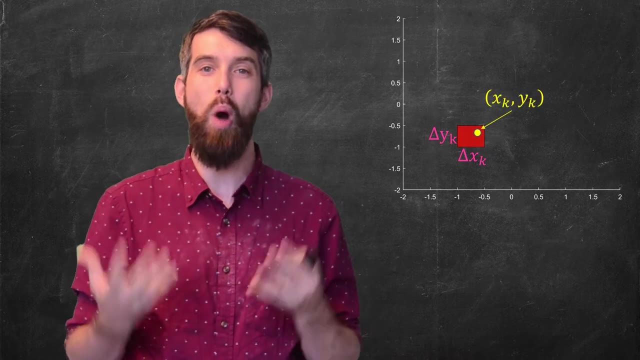 but plug what into my function? This is a whole little region. I need to choose a specific point that I will plug into my function, So let me choose a pair, a pair x k, y k, and the pair x k, y k is just some point anywhere inside of my rectangle. 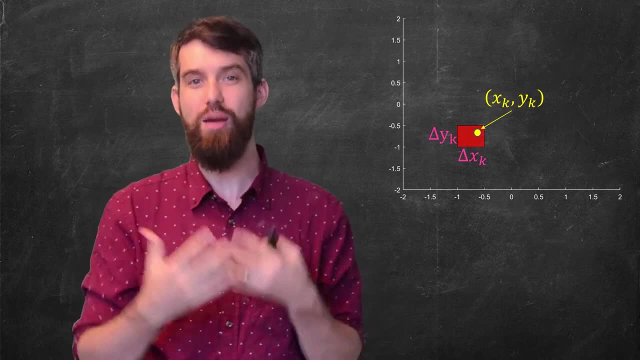 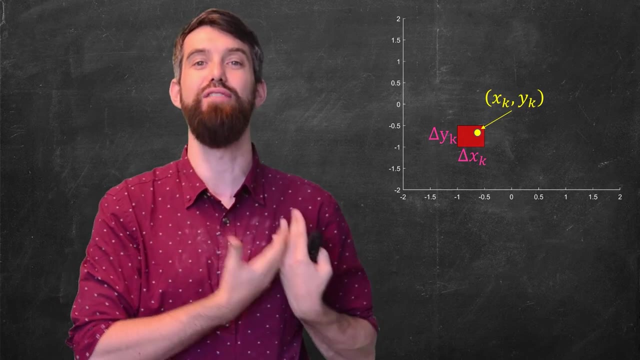 it doesn't matter. You and I can make different choices as to where that point's going to be, and well, for our approximation, our choices might matter in the limit as you go towards an infinitely large number of infinitesimally small number of these little subdivisions. 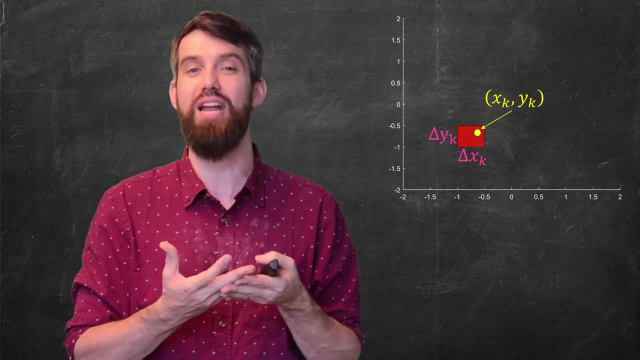 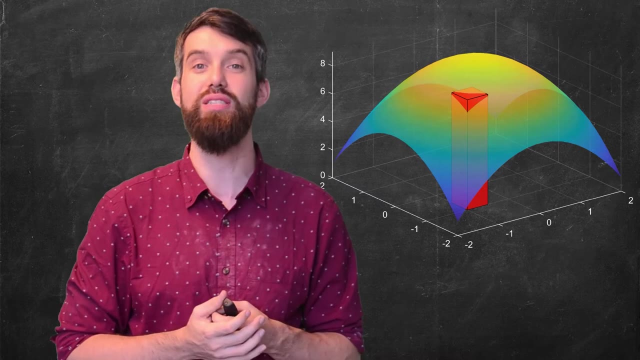 where exactly you choose the x, k, y k inside of the rectangle is not going to actually matter. So that's the domain. Now, if I go back and look at what it looks like for the graph of the function down the base, I have that delta x k and delta y k. 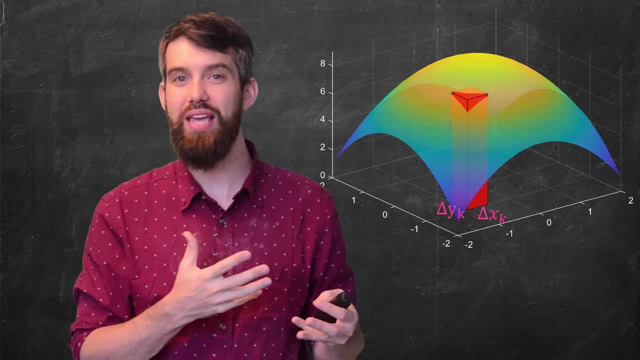 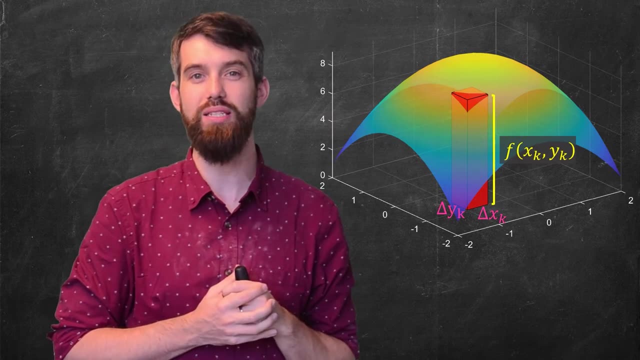 and then, if I take that specified point, the x, k, y, k, if I take f of it, f of that point is going to give me the height of my particular box, And so the volume of this box is going to be well, base times height. 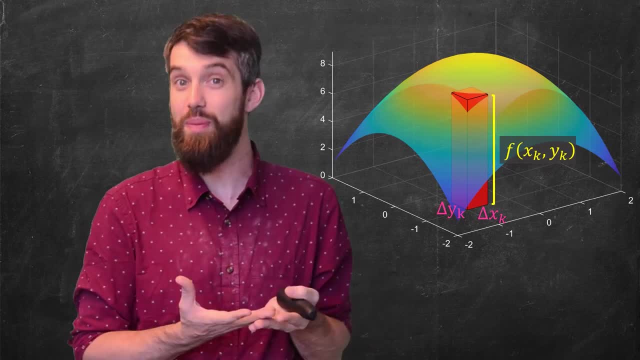 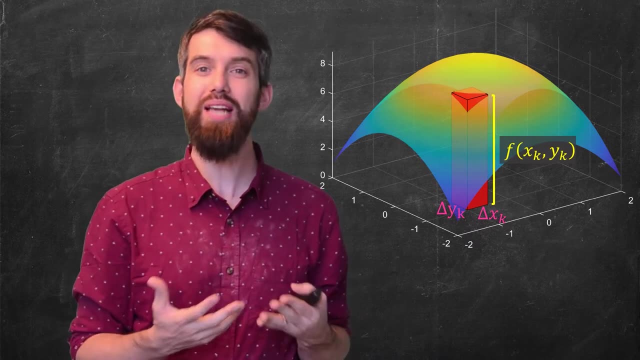 so it's the product of the delta x k and delta y k in the base and then multiplied by the height, which is the function value at x, k, y k. So the basic idea I'm going to do is I'm going to compute that volume for this one particular box. 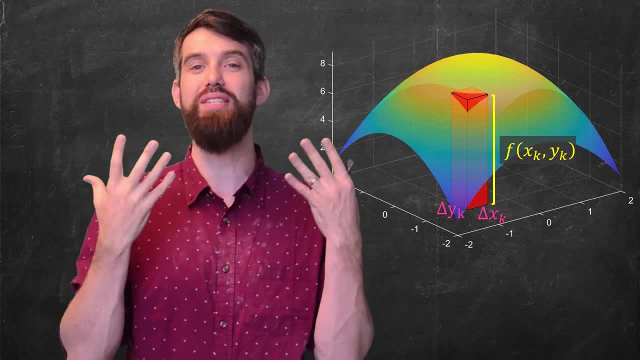 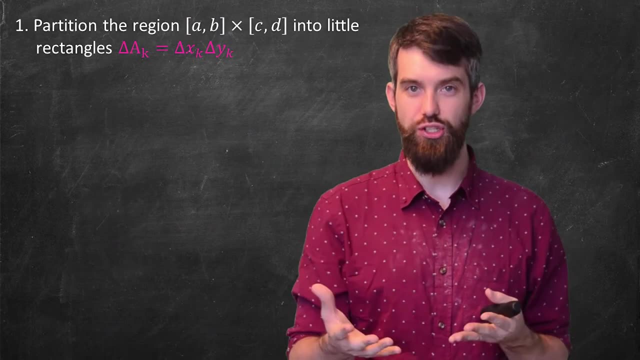 then I'm going to add it up over all of them and finally I'm going to take a limit in some sense. Now let's see how we do this more properly. So the first thing I'm going to do, if you give me a region, 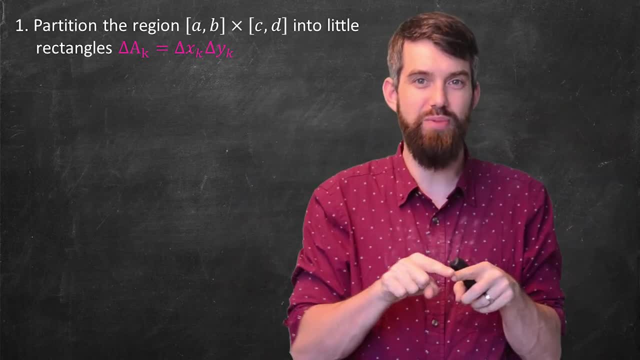 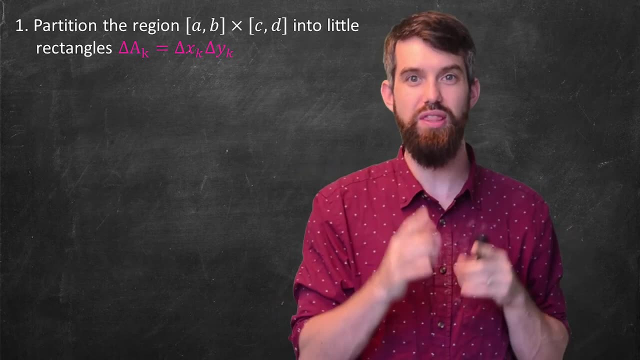 and, by the way, for this video, the region has to be a rectangular region, a region where it's just a change in x and a change in y. but if you have such a region, then the first thing that I'm going to do is I'm going to break it up. 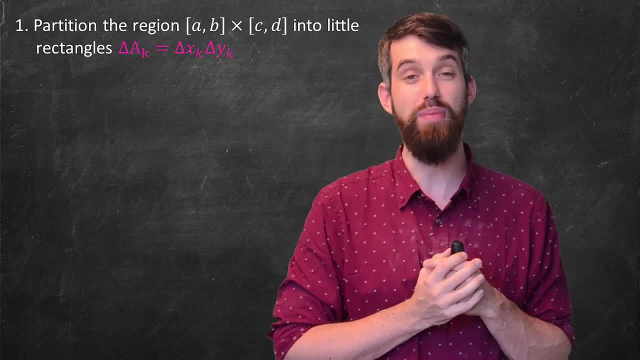 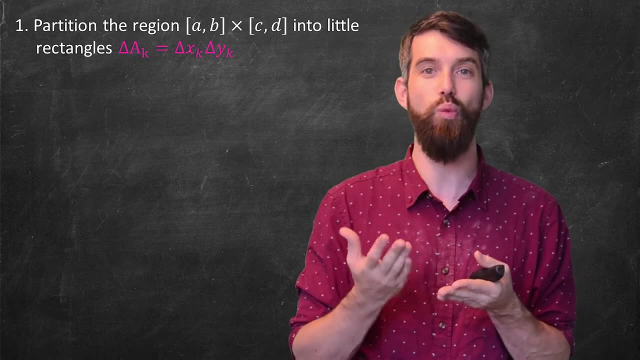 I'm going to partition it into a bunch of small little rectangles, And the area of each of those rectangles is going to be given by the product of the change in x k times the change in y k. So the total little area that I have is this product of these two things. 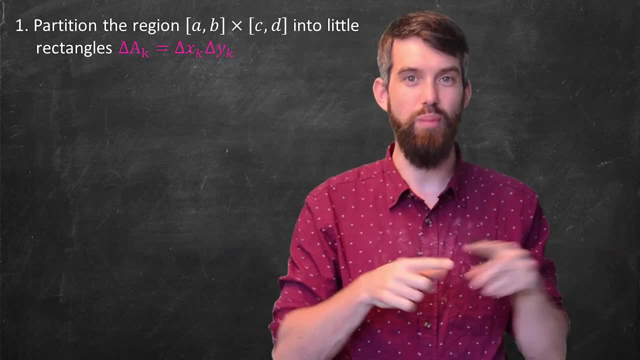 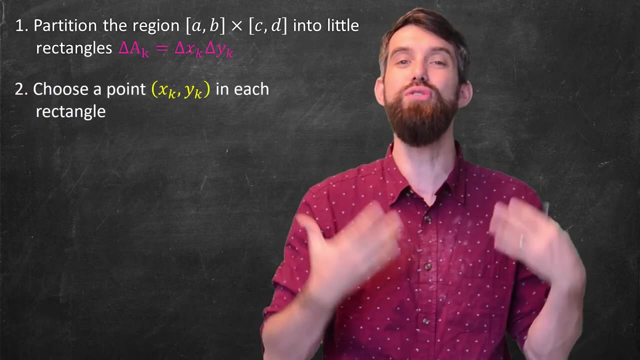 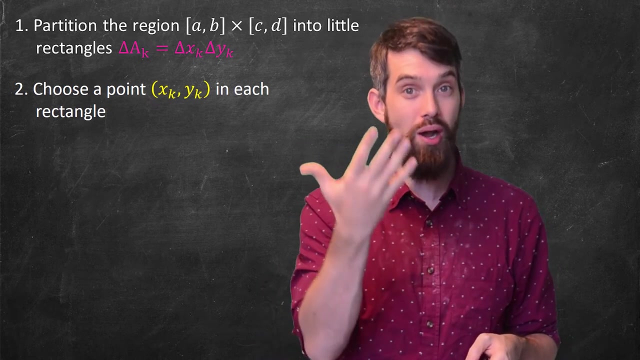 Then if I take this rectangular region which is broken up into a whole bunch of little rectangles, in each rectangle I'm going to choose some particular point. So I'm going to choose an x, k, y, k inside of each of my little rectangles- Then if I want to approximate the volumes- this is not exactly the answer. 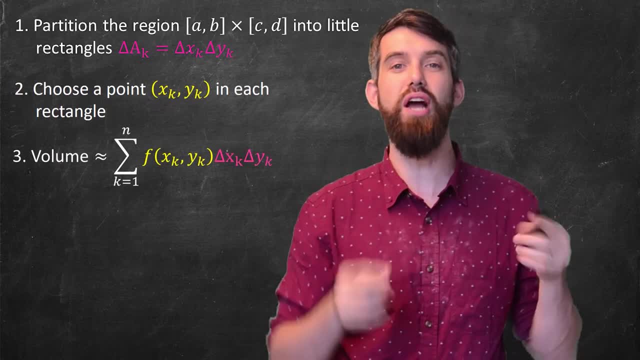 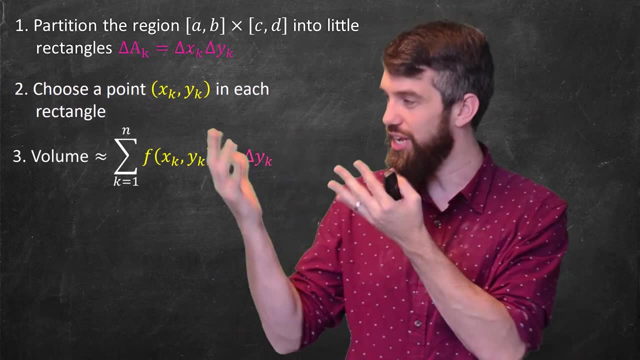 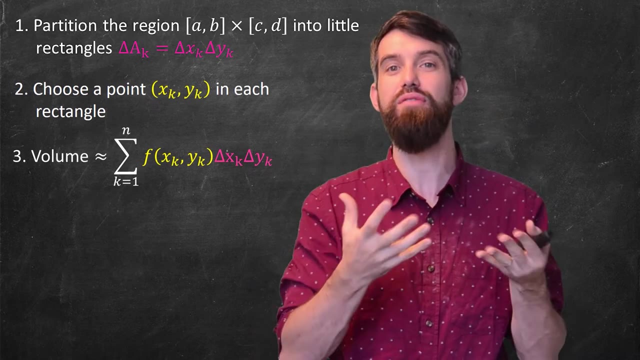 but if I'm going to do an approximation, if my partition of that big rectangular region into n different small little rectangles, then I will take the sum. that's what this notation means. sigma is the sum from 1 up to n and I'm adding up the sum of all the volumes of these little boxes. 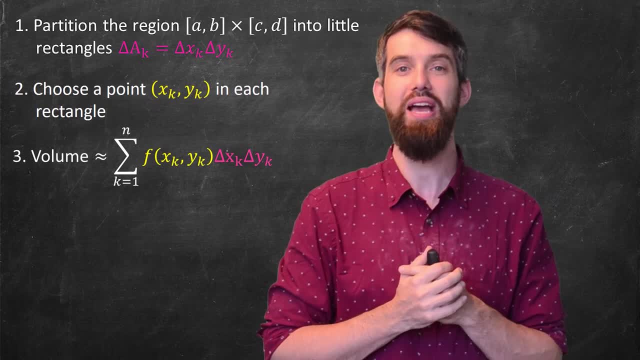 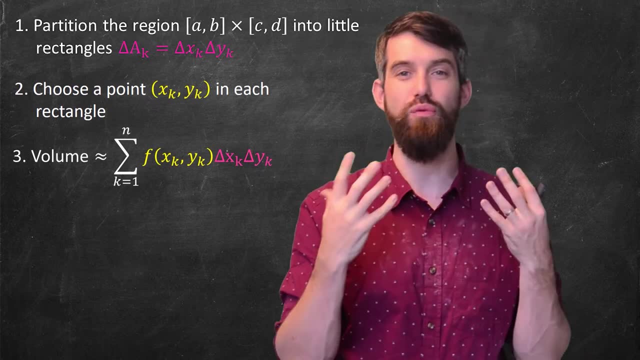 where the heights are given by the f of x, k, y, k and where the widths are given by the delta x, k, delta y k. Then comes the real magic of Riemann integration. This volume is an approximation, but what I'm going to do is I am going to define this. 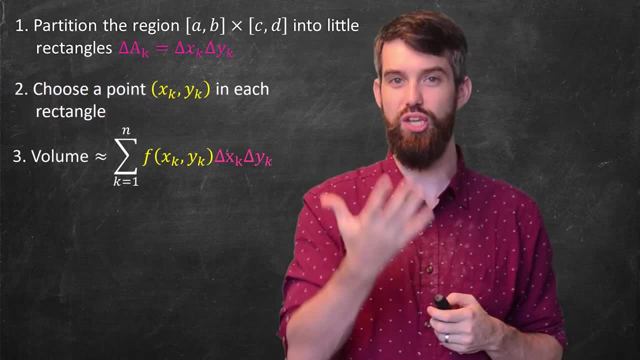 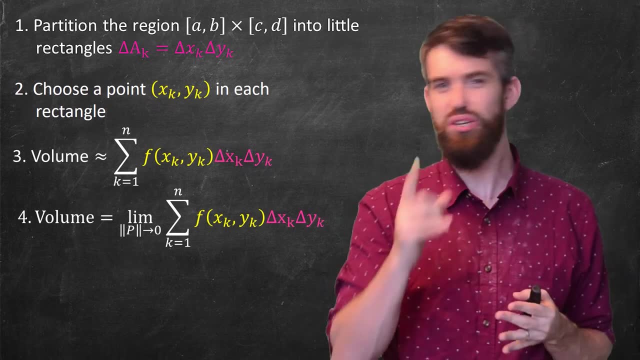 I'm going to define the volume under this region by talking about a particular limit. I'm going to define the volume to be equal to a limit, as the length of p goes to 0, we'll talk about that, of this sum from 1 up to n, of all of these little volumes. 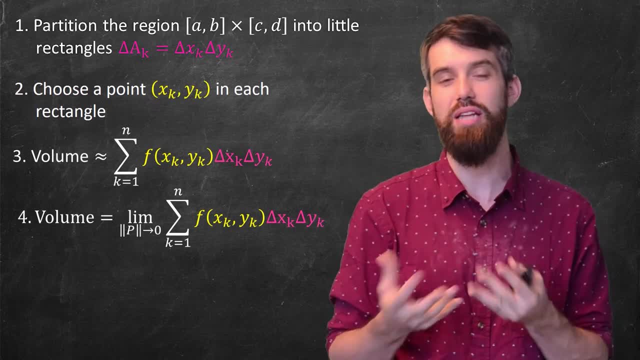 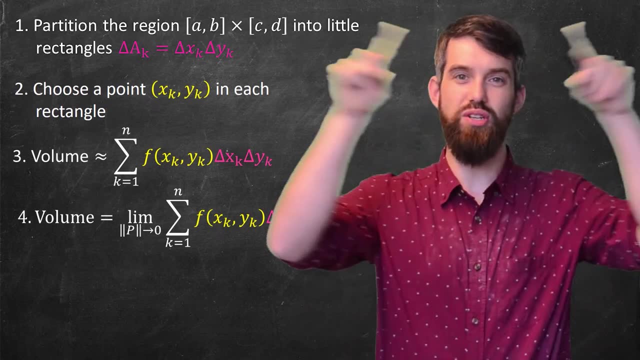 the f of x, k, y k times the delta x, k, delta y k. And then what is the limit doing? Well, p is just the name I give for this partition where I took this big region and I partitioned it into the sum of a bunch of little rectangles. 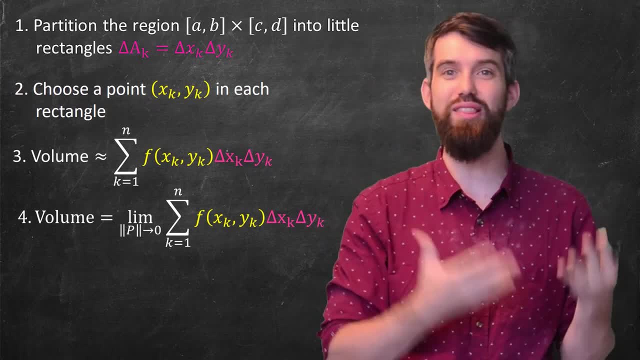 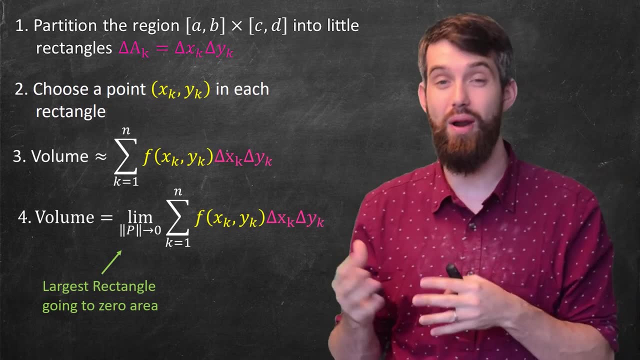 And when I take that the length of p goes to 0, well, what I just mean by that is that the largest rectangle in that partition- some might be bigger, some might be smaller- I'm saying the largest rectangle is going to go to 0 area. 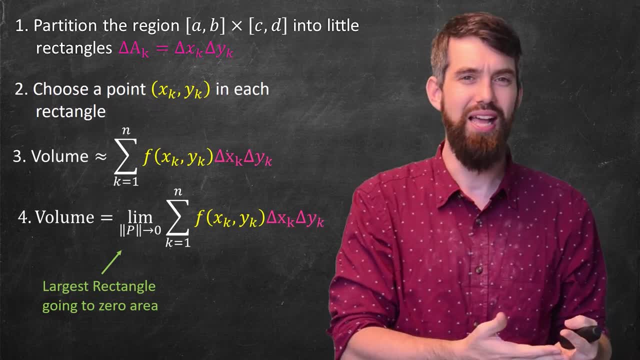 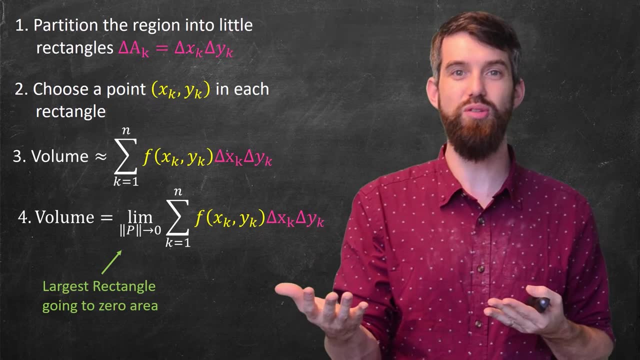 which means all the other rectangles are going to go to 0 as well, And indeed, if the area of these rectangles is going to 0, what we're meaning is that the number of those rectangles is going to infinity. So there's many different ways to talk about this limit. 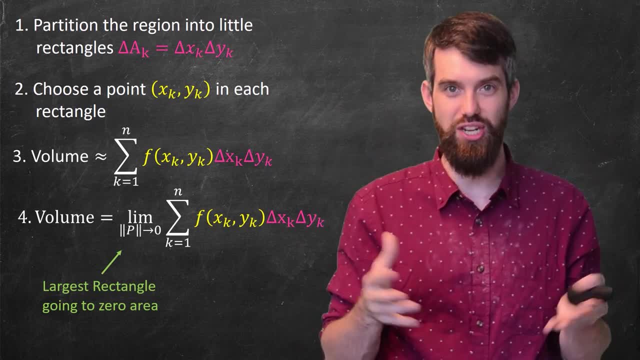 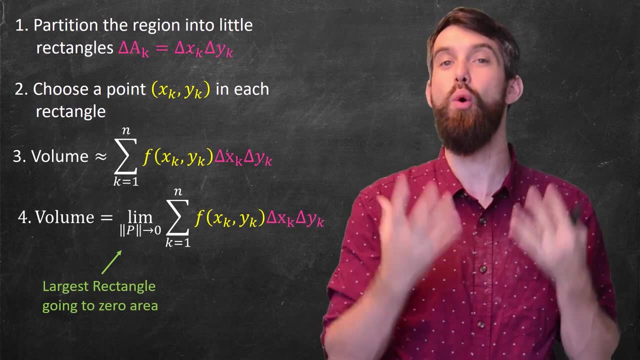 which means I'm getting a better and better cutting up of my region into a finer and finer partition where the maximum size of any individual, a k, is going to 0 and the number of them is going to infinity. Nevertheless, I take that limit that I'm trying to describe. 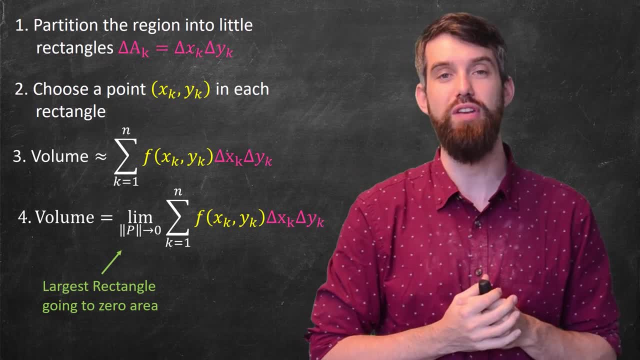 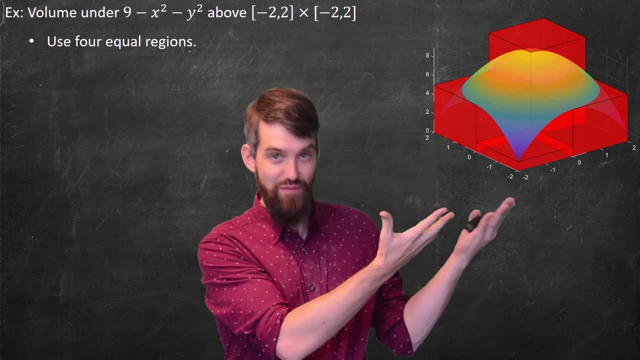 I take that limit for this particular sum and that's going to be my definition of volume. Let's see an example. The first thing I want to do is consider the same function that I've been talking about- 9 minus x squared, minus y squared- and on the same region that I plotted here. 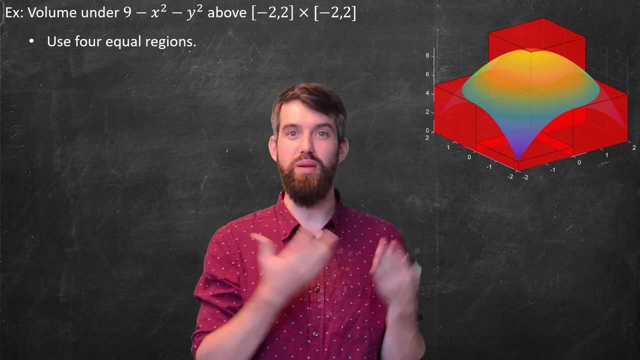 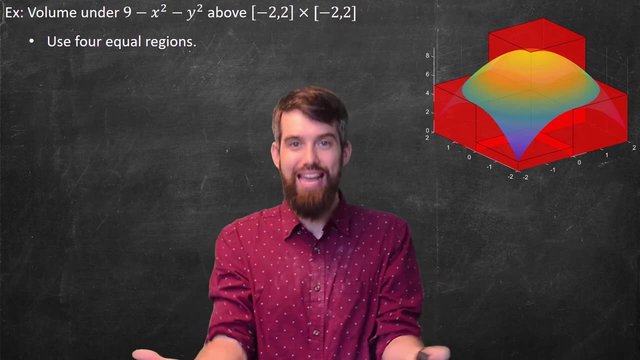 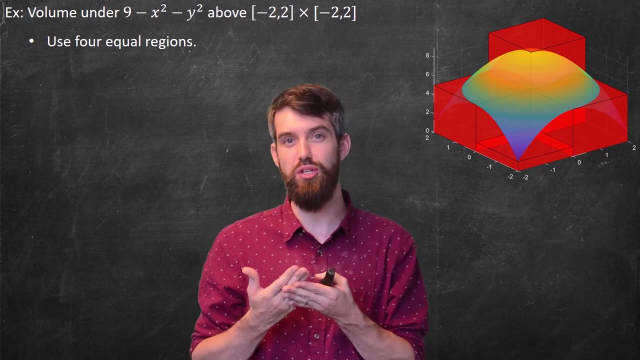 So the x is between minus two and two and the y is between minus two and two. The way I represent this is using one interval times another interval. That's my notation for talking about a region that bounds the x and the y. So the x between minus two and two and the y between minus two and two. 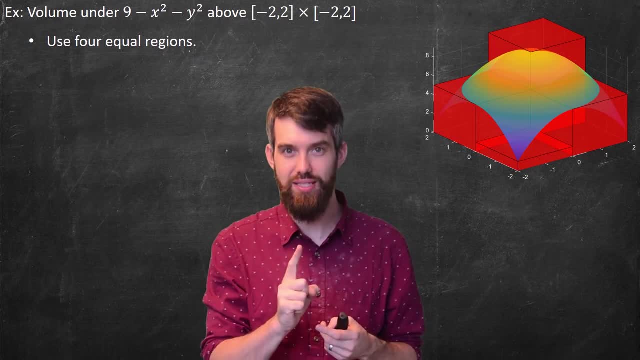 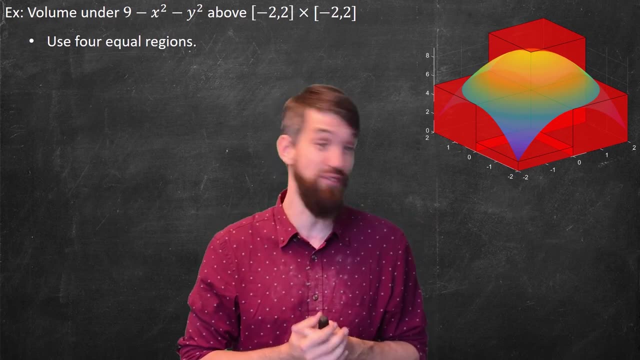 Then the next thing I'm gonna do is I'm going to go and approximate this by just four rectangles, And the reason I'm choosing only four rectangles is I want it to be something that we actually can compute out of this video, not 18, or any other number. 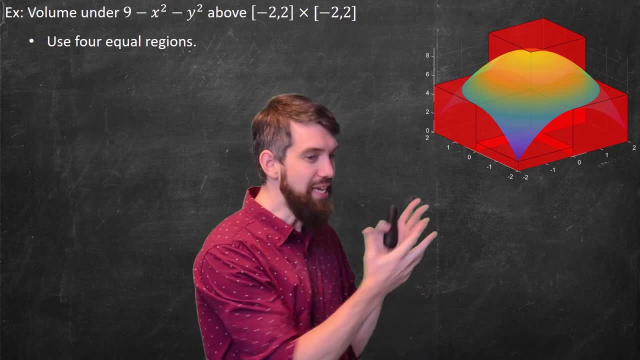 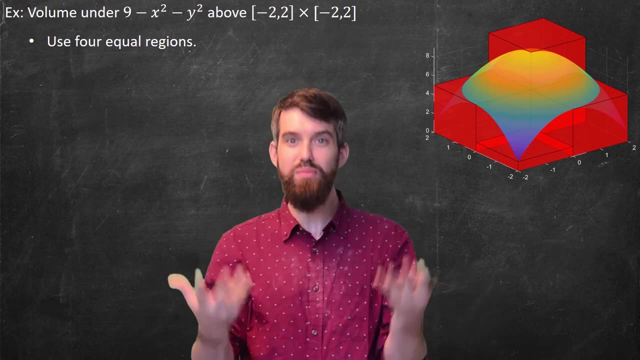 But for 4 rectangles we have a 1, 2, I think we can compute it. So what you see in the graphic here is these four different boxes, each of different heights, and my approximate volume is going to be the sum of the volumes of 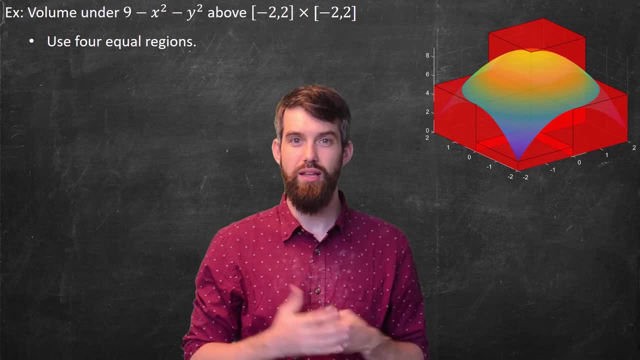 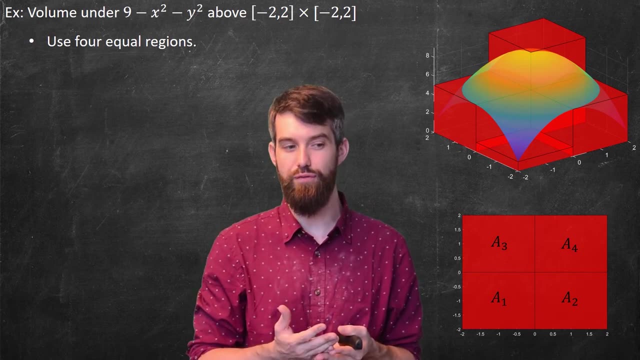 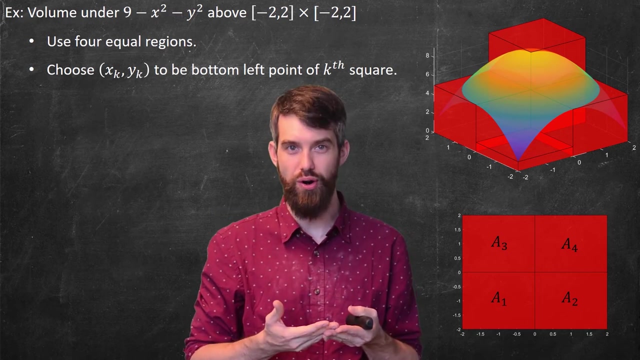 those four boxes. If I focus in on the domain, then what I'm going to have is these four little rectangles, and a1 and a2, and a3 and a4, and I'm going to make a specific choice. I'm going to choose the xk- yk to be on the bottom left corner of these four different boxes. So in other words, 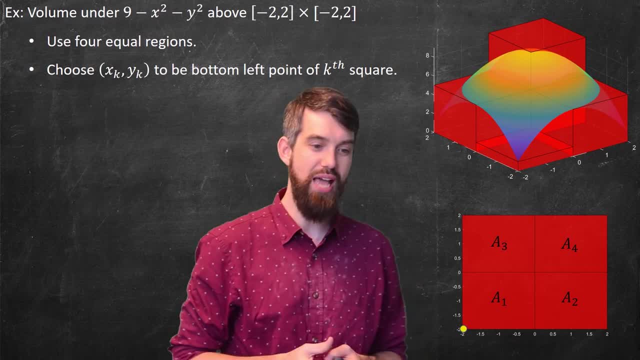 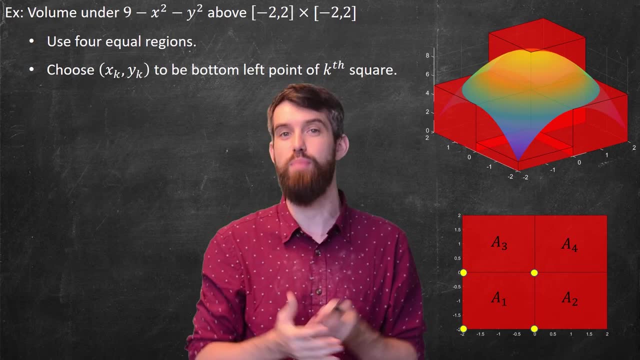 for the a1, the specific choice that I'm going to put down here is the point minus two, two. and then for the a2, the a3 and the a4, I can just put these other four points always at the bottom left corner. Could have chosen the top right corner, or choose in any corner, but for this approximation that's. 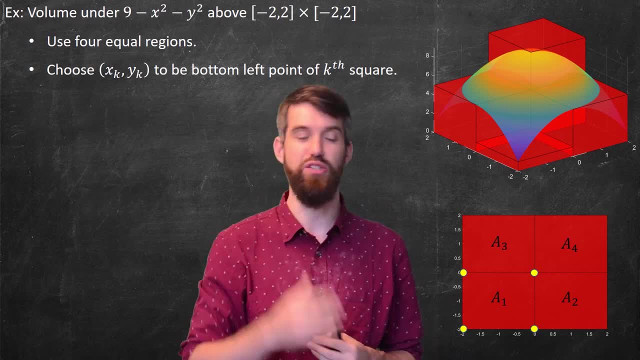 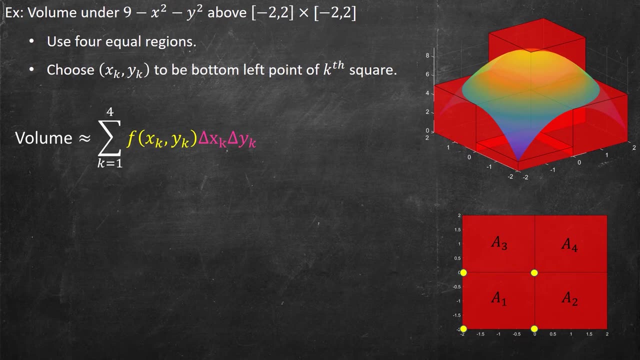 the corner I'm going to choose Now. I'm going to step away, because there's going to be a bunch of formulas on the screen. Then what I want to do is I'm going to say my volume is going to be is approximately equal to the sum of four things, these four different boxes. 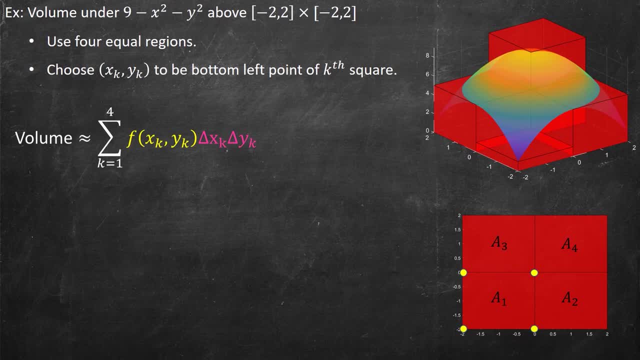 these four different rectangles with heights above them, and that those heights are going to be given by the function value of the four points that I've chosen multiplied by the delta xk, delta, yk. Well, in this example, the change in the x and the change in the y for any of those four little rectangles. 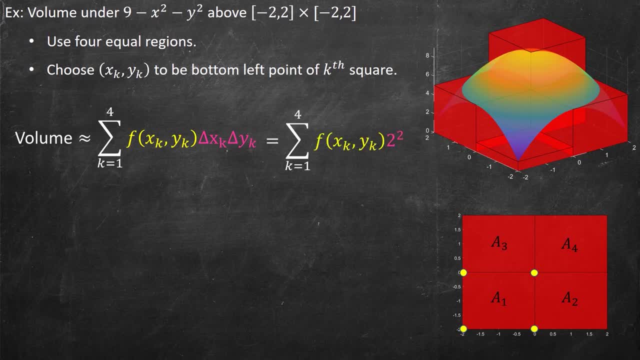 is just 2.. So this is nothing but the sum of the function values times 4, times 2 squared. I'm going to evaluate this function at the four different points. So evaluate the function of minus 2, minus 2, 0, minus 2, minus 2, 0, 0, 0.. Those are the 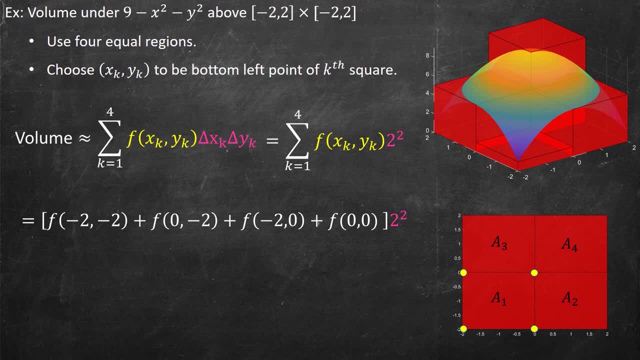 four different points and each of them gets multiplied by this 2 squared. If I just plug those into the function, I get 1 plus 5 plus 5 plus 9 multiplied by 2 squared and that's going to give me a value of 80.. So this is an approximation. 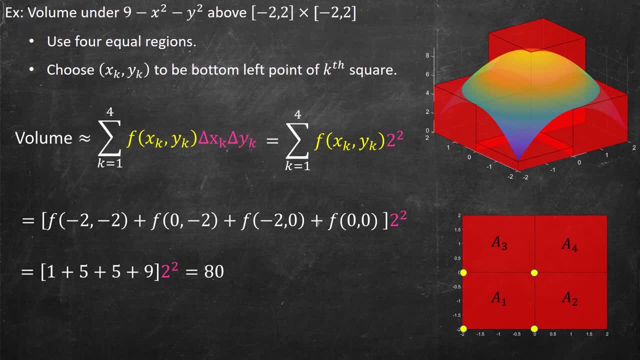 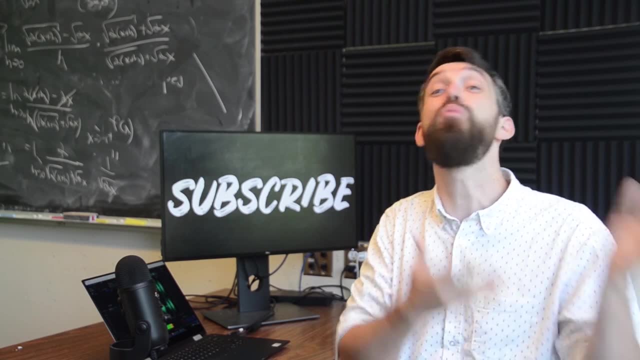 to the area under this particular surface. If you have a question about this video, leave it down in the comments. We're all mathematicians here. we appreciate algorithms, so let's just help the YouTube algorithm out by giving this video a like. and finally, if you